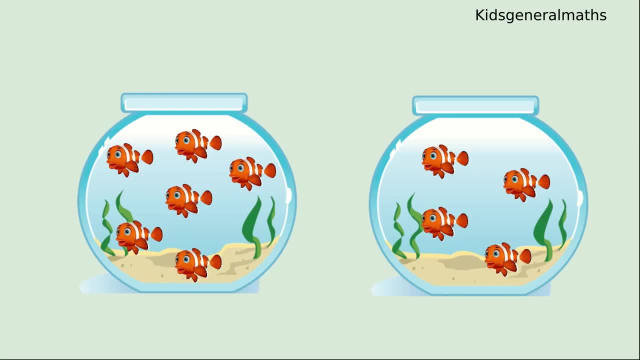 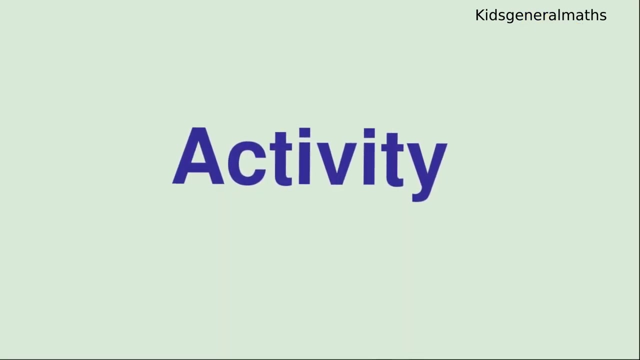 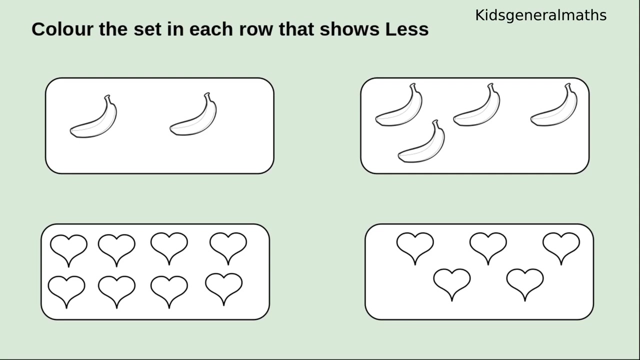 four, five, six. The first pot has six fishes: One, two, three, four. The second pot has four fishes. While comparing these two pots, six is more, four is less. Next, we are going to do some activities. First, we are going to count these objects and we are going to color. 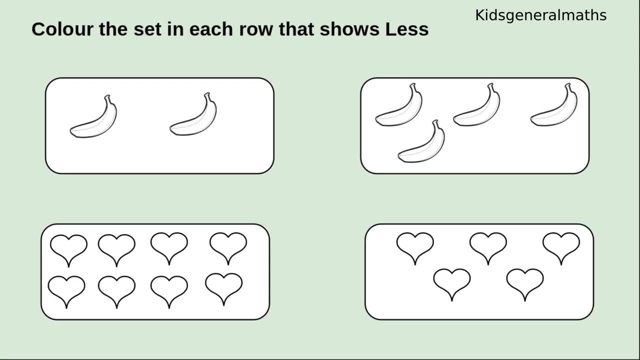 which is less. So first we are going to count the first boxes: One, two. So this boxes has one, two, three, four. The next box has four bananas. While comparing this two numbers, which is less, two or four? Any guess? Yes, two is less. So we are going to color the. 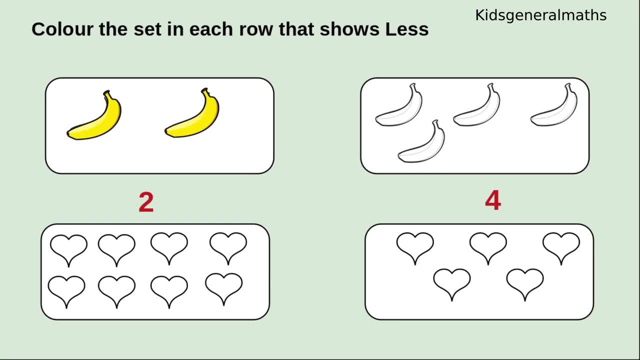 two bananas. Next, we are going to color the heart shape, which is less One, two, three, four, five, six, So these two are less One. two, So this box is less. Next, we are going to color the banana, So this box is less. Next, we are going to color the banana, So this box. 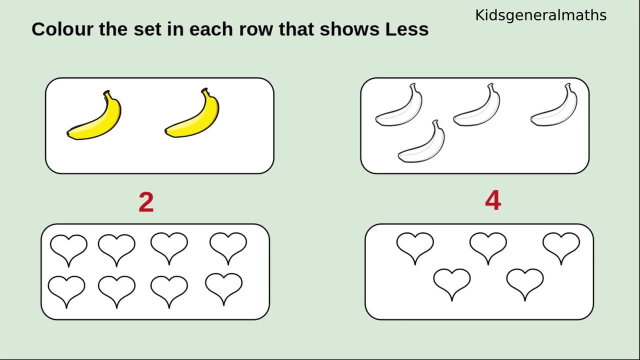 6,, 7,, 8.. So this box has 8 hearts: 1,, 2,, 3,, 4, 5.. This box has 5 hearts, So we are going to color which is less, 8 or 5.. Well, comparing these two numbers, which is less? 5 is less. So we are going. 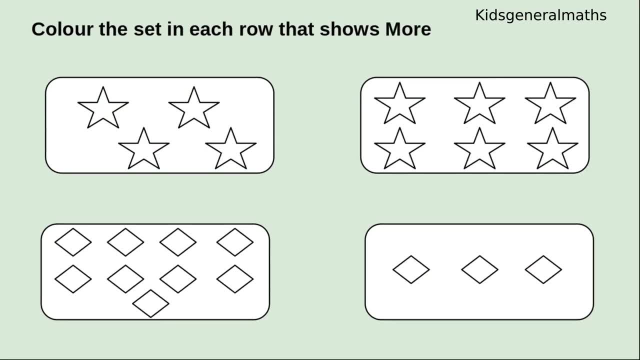 to color it. Next we are going to color which is more So in the first two boxes: 1,, 2,, 3, 4.. How many stars? 4 stars. So the next two box has 1,, 2,, 3,, 4,, 5,, 6.. How many stars? 6 stars, So we. 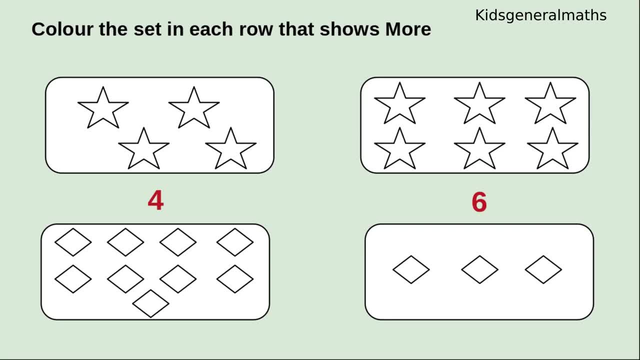 are going to color which is more So, while comparing this two number: 4 and 6.. Which is more? Yes, 6 is more. So we are going to color the 6 stars. Next, they are given diamond. We are going to color which is more: diamond: 1,, 2,, 3,, 4,, 5,, 6,.